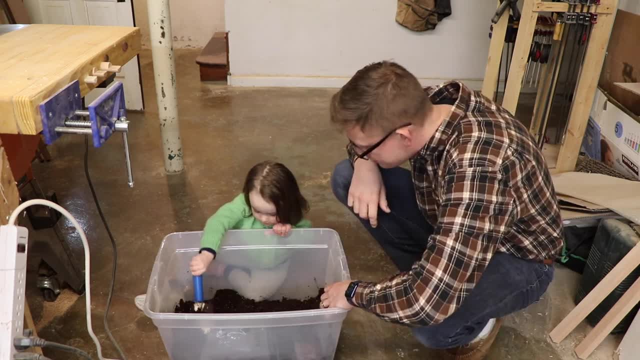 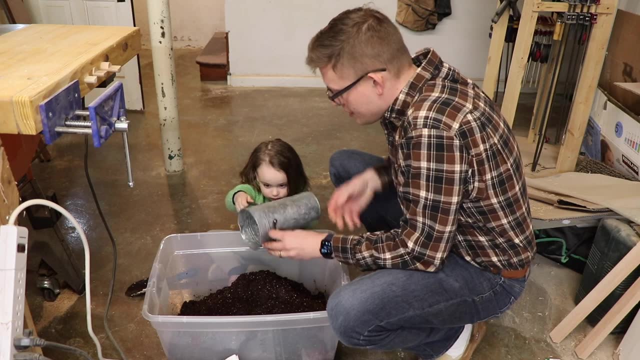 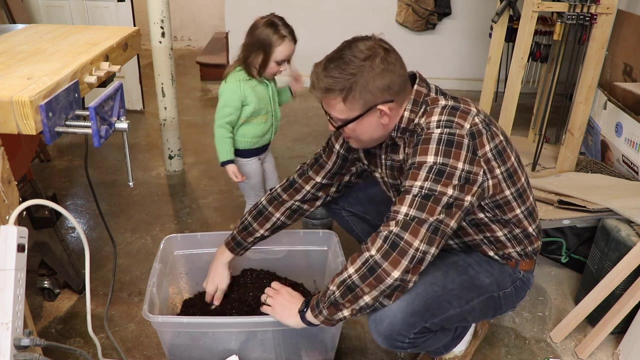 got to be good, It's got to be nicely mixed. Yeah, There, Good. Will you hand me that please? Okay, Okay, Thanks, And then we mix it all together. I'll pour this until you get more water, Thank. 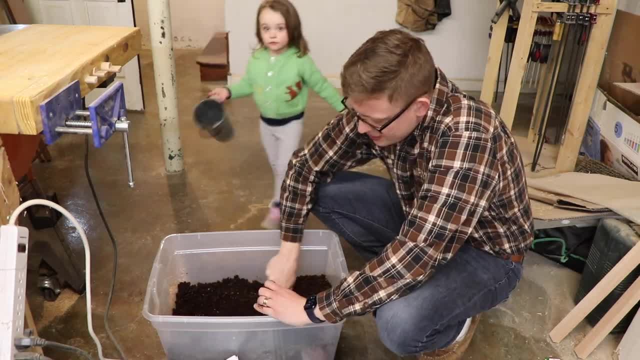 you so much. Charlotte is two and a half years old, and she remembers being in the garden with me last year Already, when she was just one and a half years old. she was like: I'm going to make this, I'm going to make this, I'm going to make this, And we were putting 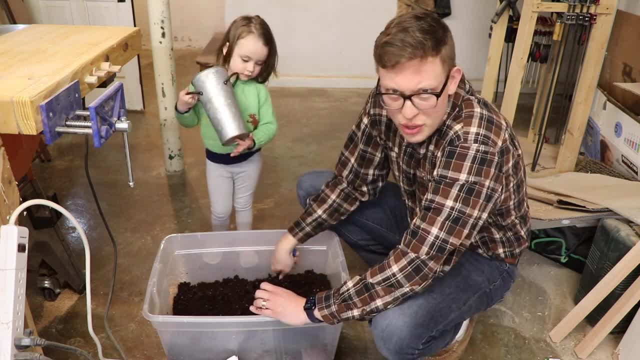 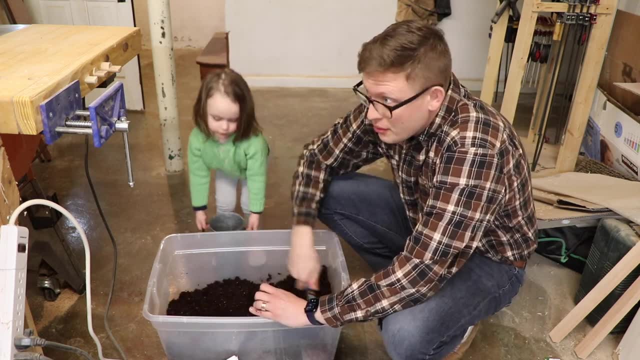 seeds in, like bean seeds and squash seeds, something real big that she could understand. I'd dig the hole and she'd plop it in and we'd pat it down together And this year we're upgrading to seed, starting inside to get the year rolling And you're excited about. 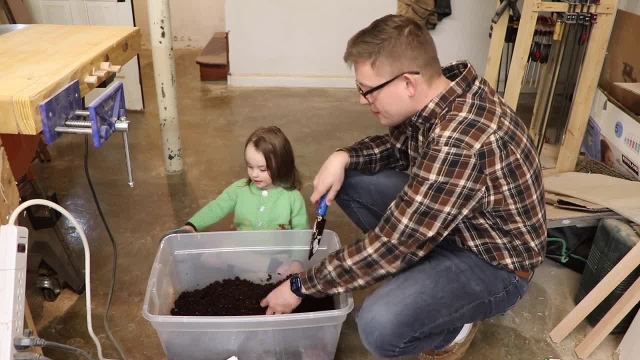 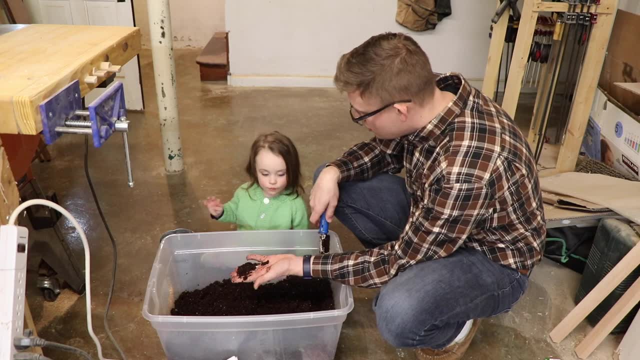 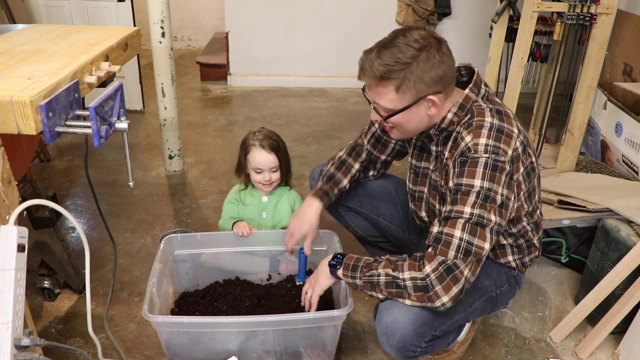 this, aren't you? Yeah, What do you think? Here, I've got this mixture and it forms a nice ball and then it breaks apart. I think that's good, don't you? Yeah, How's that? does it smell delicious? that's the word. all right, Charlotte, I'm going to take. 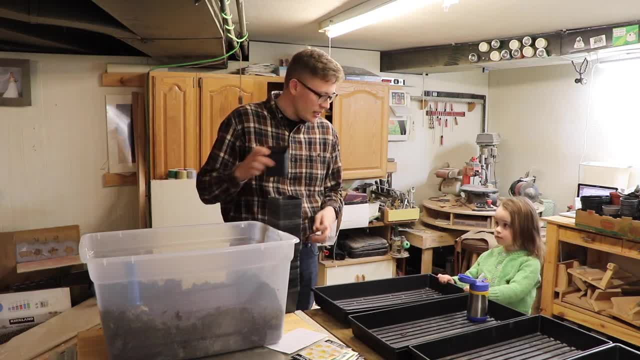 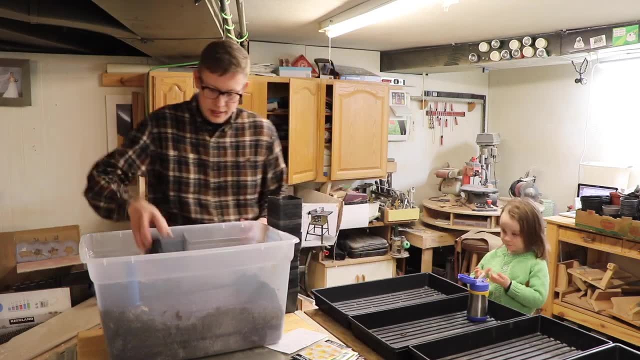 all of these little trays, and I'm going to be filling them up with soil, and then you're going to help me put them in rows. okay, sound good, let's get started. so now we're filling these up with the soil that the plants are going to grow in. 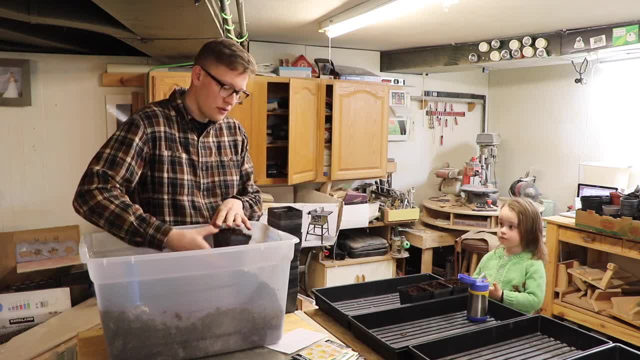 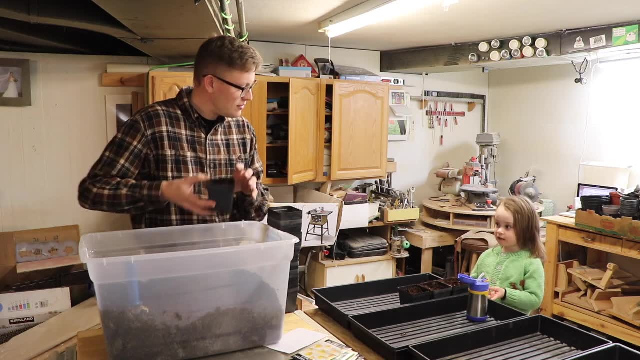 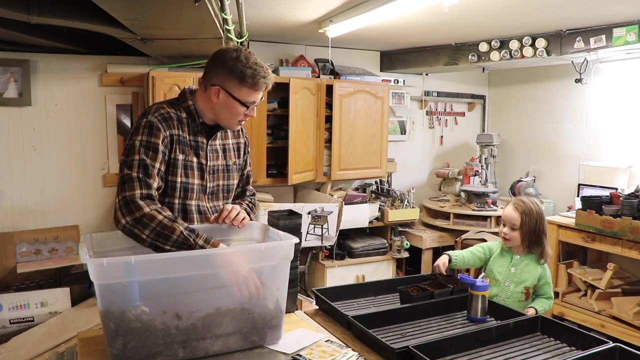 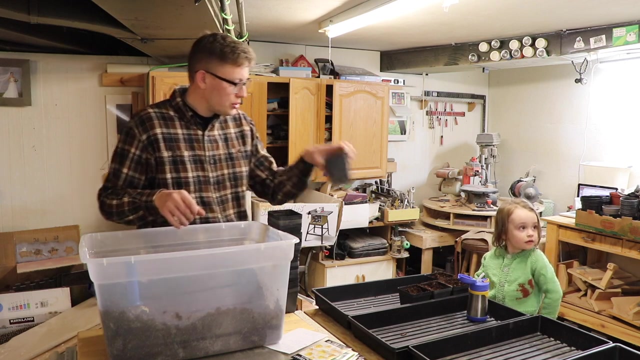 this gives enough space for roots to form. do you know where roots are? what are roots? well, you were right that roots are long things. roots go deep into the ground. they help plants take up nutrients from the ground. they help plants take up nutrients from the ground. they help. 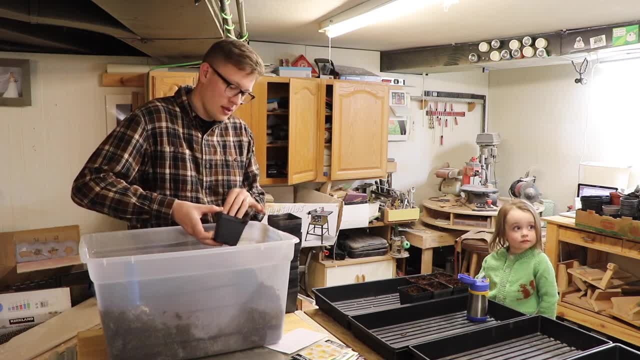 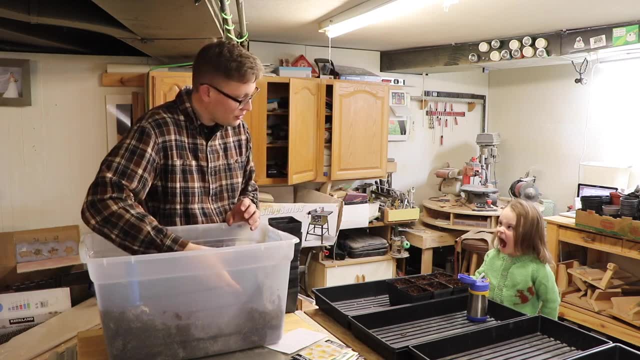 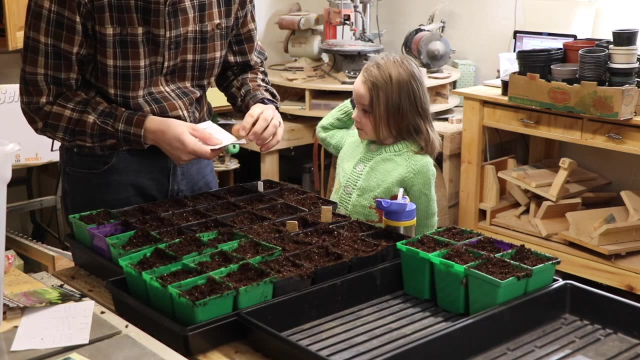 the soil nutrients that they need to grow. So by giving the roots enough space to form, we're making sure that the plant can get a good, healthy start to life. Gesundheit. Okay, Charlotte, Can I do one? Can I do one? You get to do the whole thing absolutely. 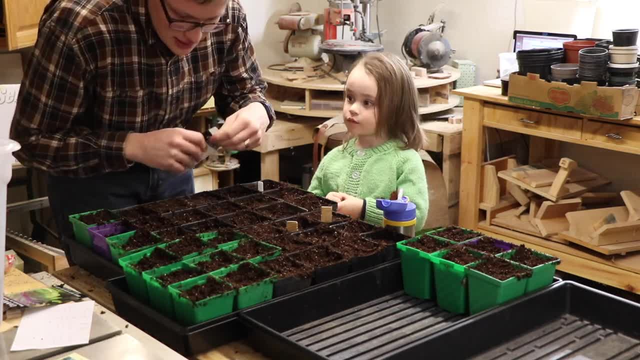 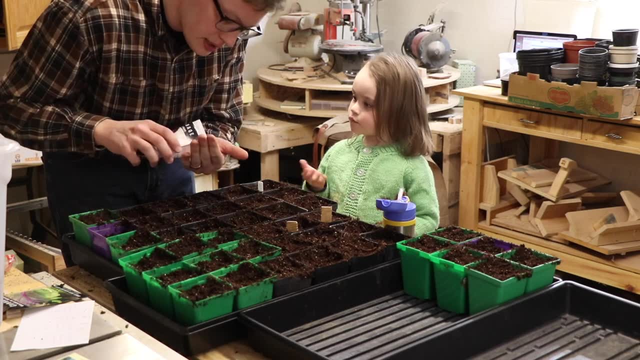 Can I do one? Yes, See, kids you want to help. Can I do one? Did you hear that? That's a wonderful thing? So we just filled 42 containers with seed starting mix and today we're planting some cabbages and Brussels sprouts. Really, Can I have some Sure, Okay, ready. 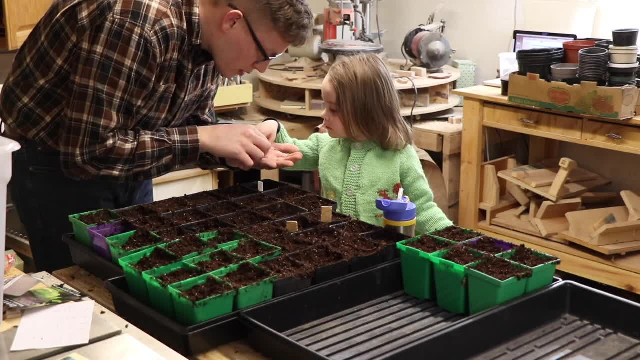 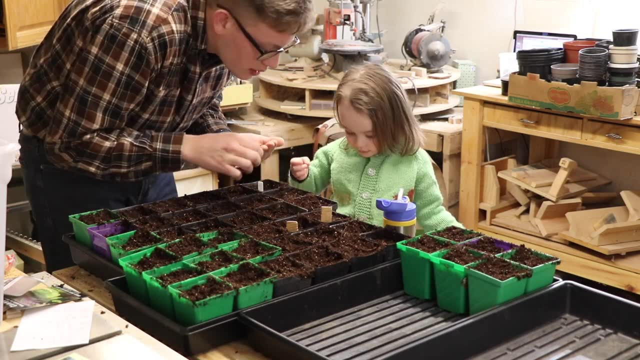 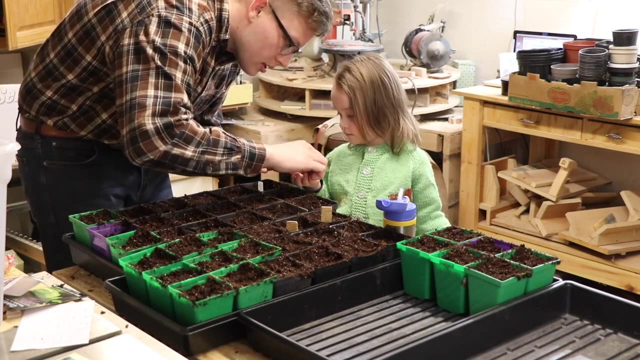 Here, See these, You feel them? They're real tiny. We're gonna put three in your hand. Ready, Hold out your hand. There's one, Put it in here, This very first one. Oh, try again. That's fine Here. Do you think you can? No, Open up your hand? Good, 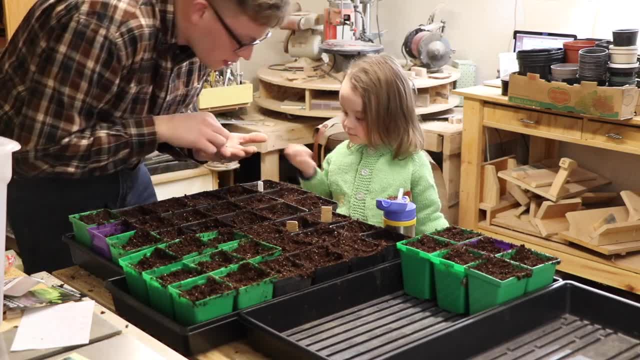 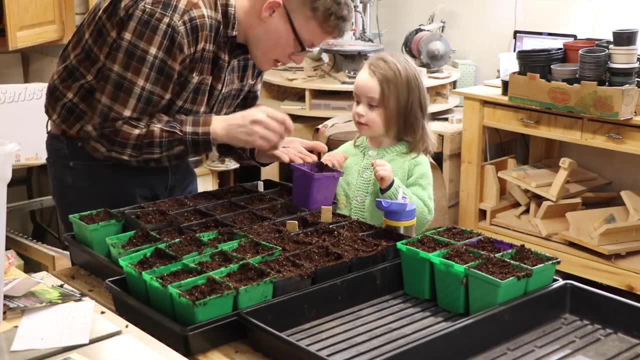 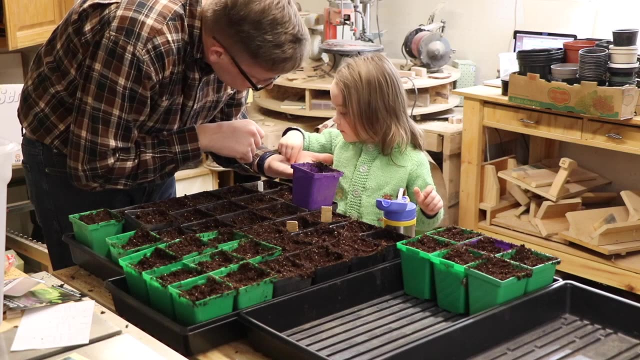 I'll put that in here. There you go. That's one, Okay, One, two, three. You want to try to pick it out of my hands? Can you pick one out of there? They're very small. You did a good job. Go ahead, Put that in. Do it again All. 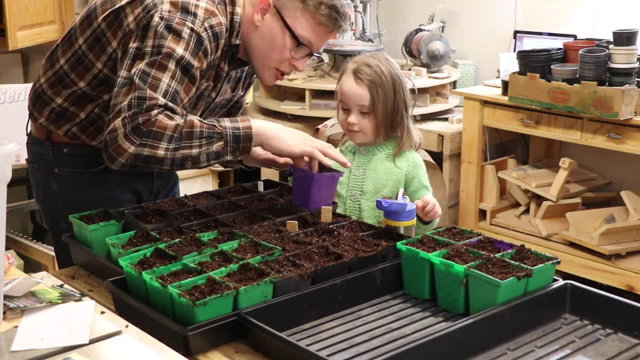 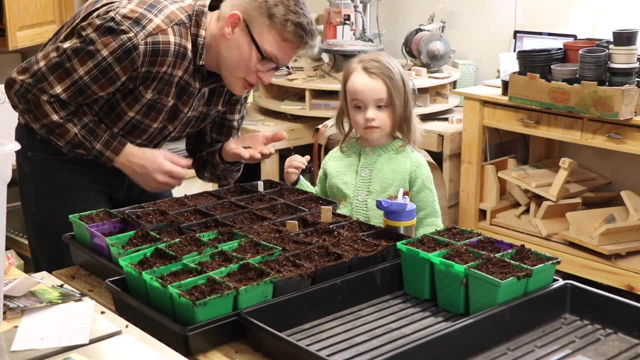 right, Okay, I'm just gonna move those around. We got more than enough in there. Nice going. See. this is discovery, not just for children but for me too, As I'm learning that her fine motor skills are getting better. she's able to actually pick these tiny, tiny cabbage. 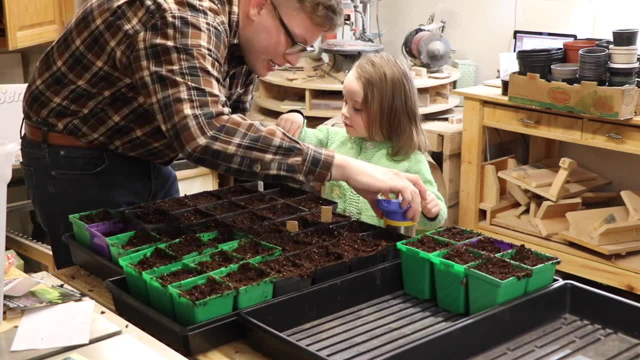 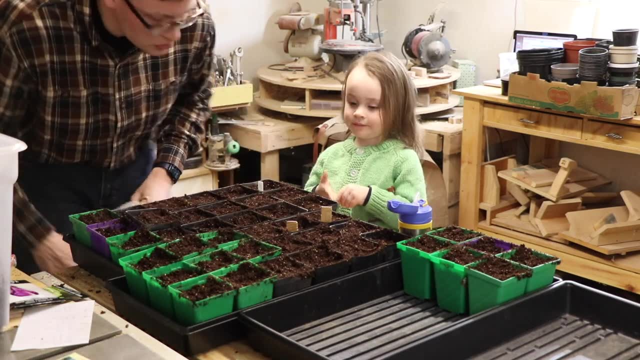 seeds by herself. Can I do it one more? Yeah, you bet. Instead of making a hole for the seeds and dropping them in when I start seeds, I just put them on top and then do an extra layer of soil. It works really nicely. 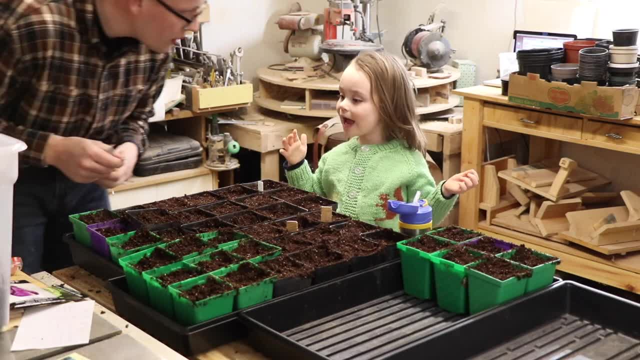 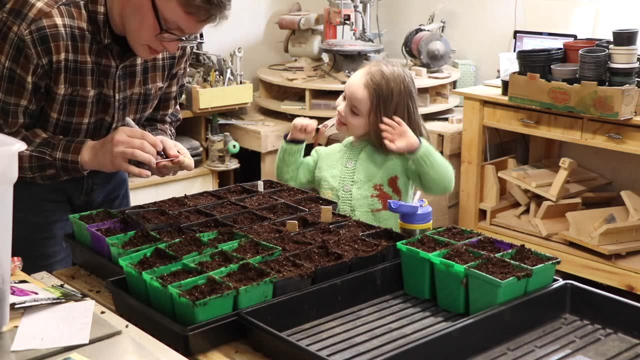 Now we're going to stick a marker in: Okay, okay, okay okay, That way we don't lose track of the seeds. This is calabose. Can I try some too? Yes, Can I try some Oh. 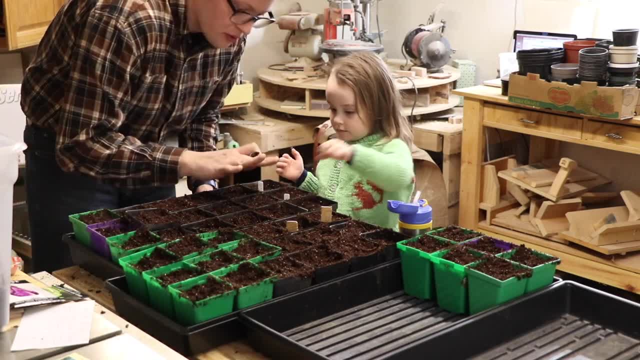 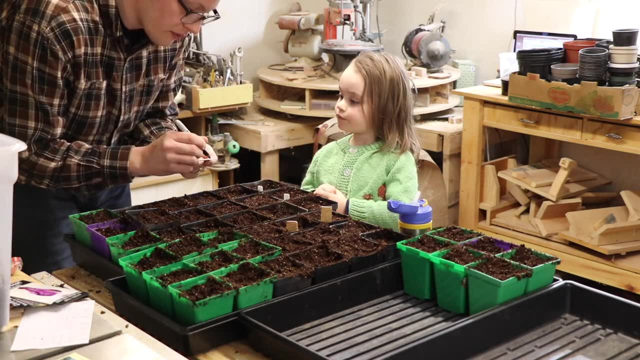 Ready? You want to stick that down? Push it down. Good, Perfect, That's perfect. right there. I'm going to, oh, leave it there. We've got to leave these inside, so we don't forget what we have. Okay, see, 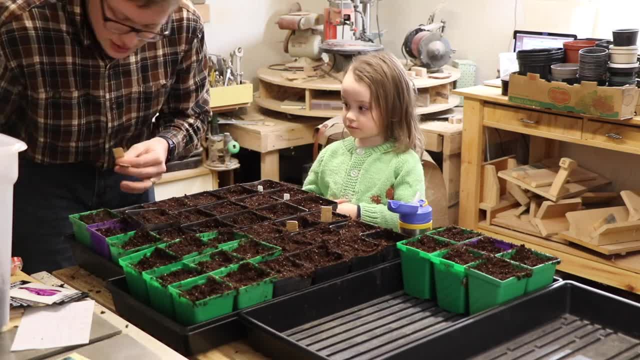 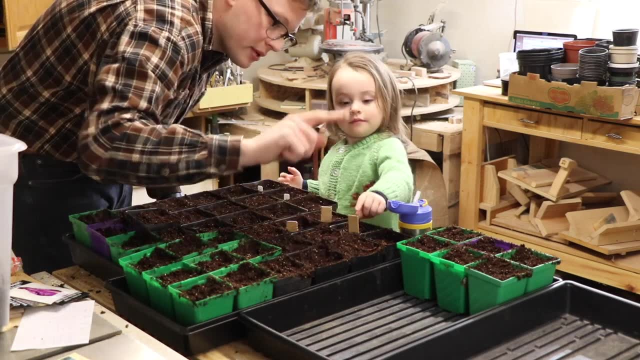 Well, sometimes we have to say no. I don't want you dealing with a very stinky, sharp black permanent marker, But you can help me shove these in Ready. Push that one down, Straight down, Good, And then we've got another one back here. if you need to do the same thing, Push it down.